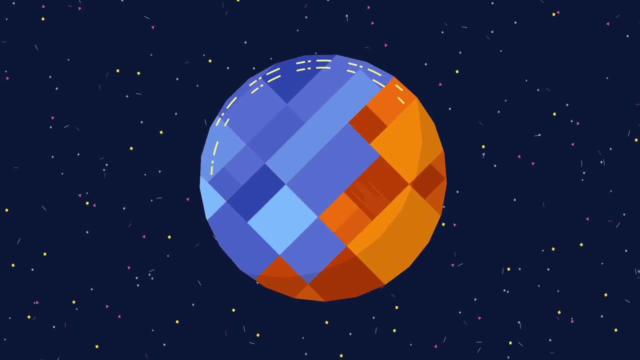 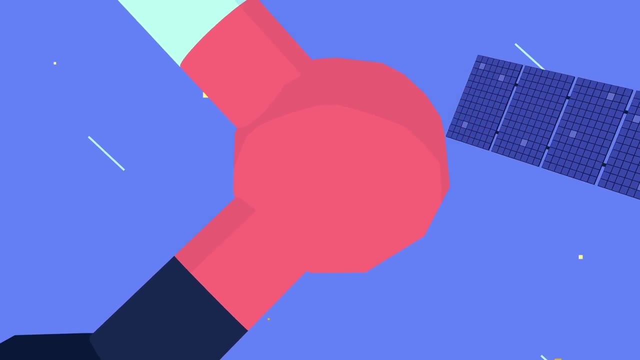 a lot warmer and wetter, resembling the Earth when life first emerged here. Mars missions have shown that liquid water used to be a source of oxygen, but now it's a source of water. The Earth is a very abundant on the planet's surface and have discovered organic molecules, the building blocks. 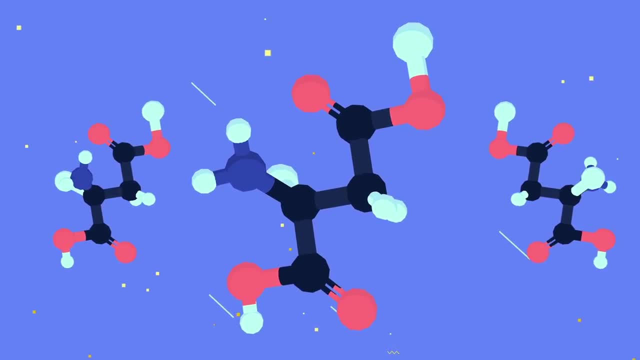 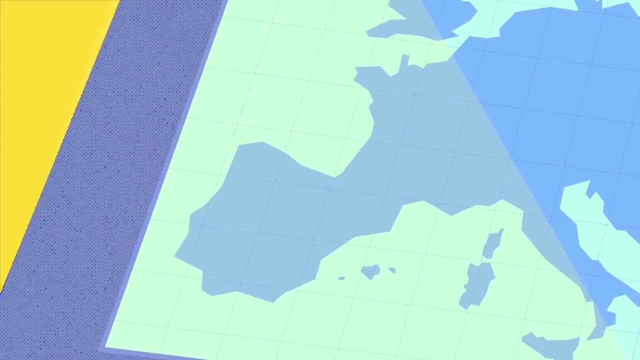 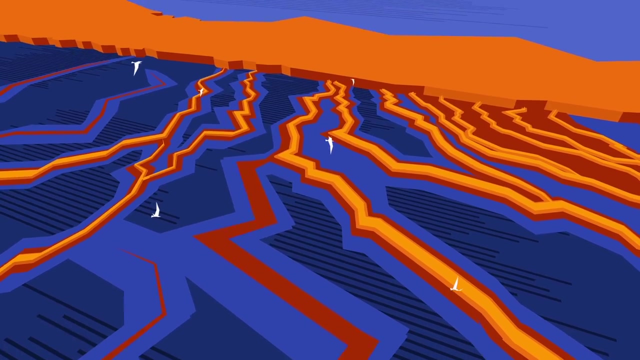 of life. Life could indeed have flourished on the red planet at some point in its history. The minerals and water chemistry in Rio Tinto in southern Spain resemble the wet environments on early Mars. This is another site scientists are using to understand what kind of life 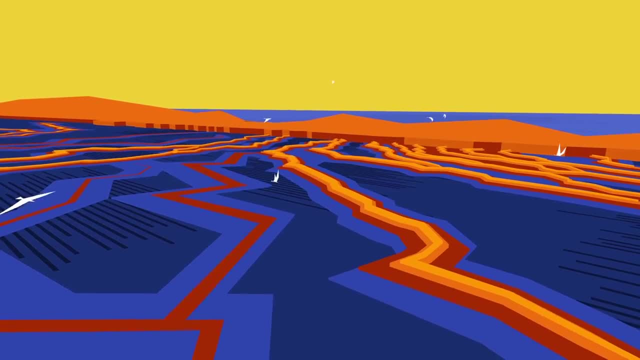 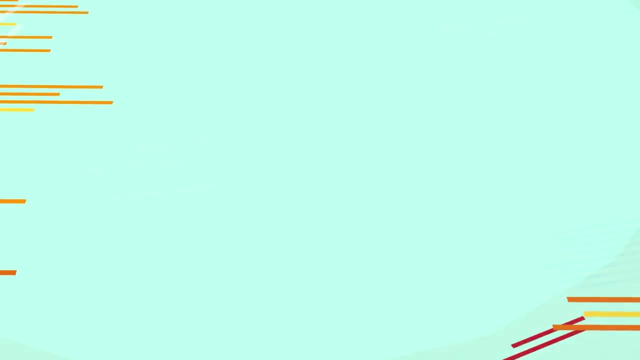 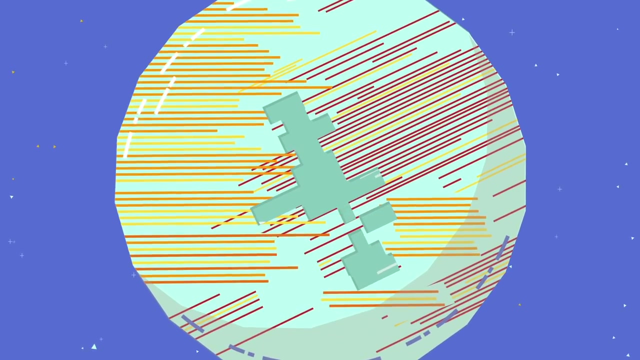 could have emerged on the red planet and how biosignatures could still be preserved. The briny Tires Lake in central Spain has features like those found in one of Jupiter's moons, Europa. This is one of the most likely locations to find life in the solar system, because it is 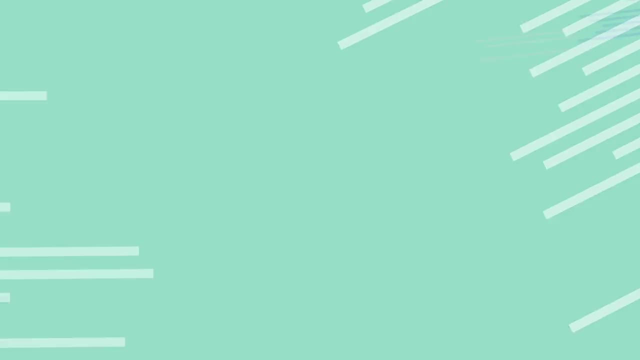 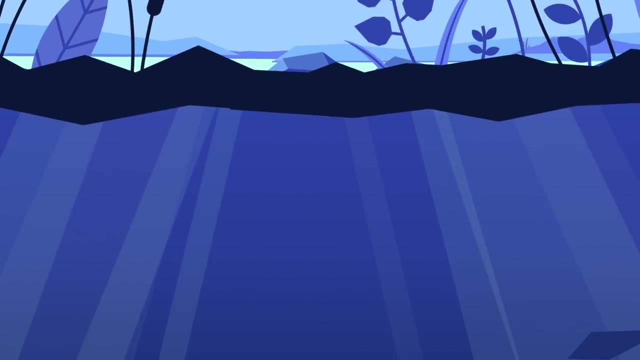 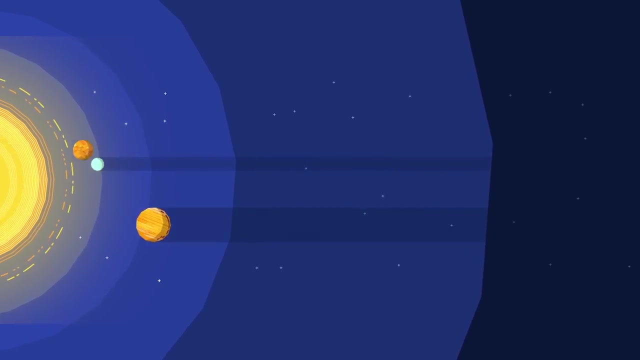 believed to have a sea of salty liquid water underneath its icy crust. By studying the extremophiles that inhabit the Tires Lake, astrobiologists can find out what kind of creatures could possibly lurk in Europa's ocean. There could also be life in the solar system, in an environment very different to anything. 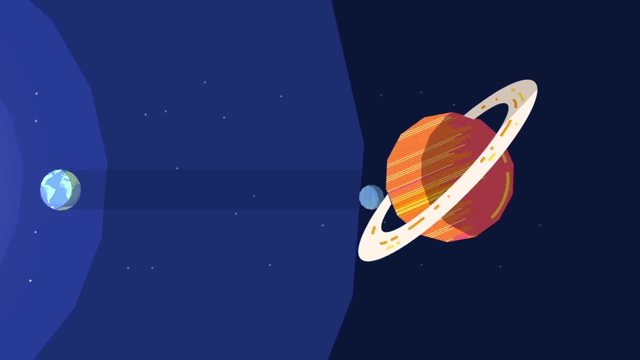 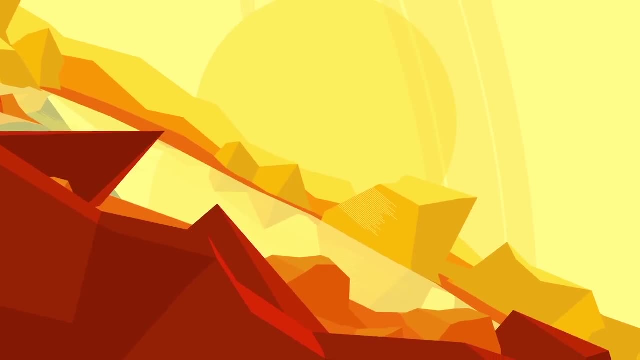 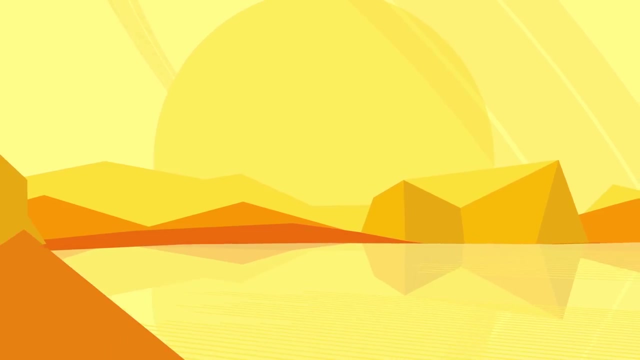 we can find on Earth. Titan, the largest moon of Saturn, is much like our planet. It has a dense, nitrogen-rich atmosphere and liquids flow freely on its surface. However, Titan's lakes, rivers and seas are made of liquid hydrocarbons- methane and ethane- Any life existing on the surface. 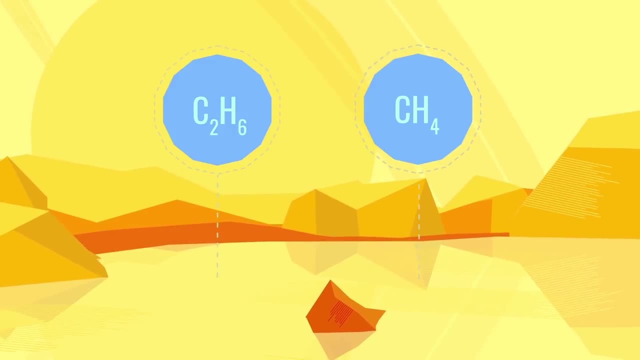 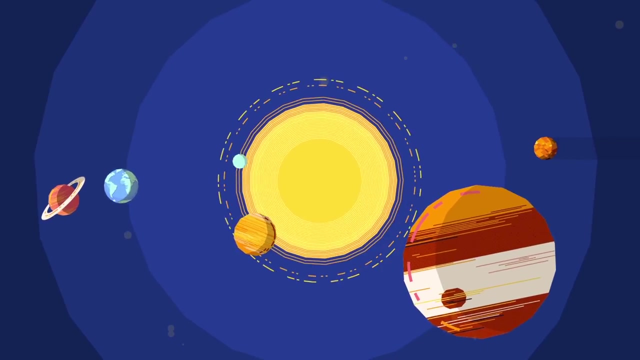 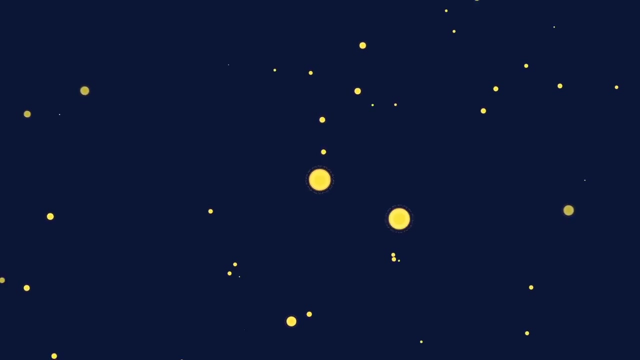 of this moon would need to use these ж solvents in place of water, an exotic chemistry compared to organisms found on our planet. Life as we know it could well be found outside our solar system. Over the past two decades, astronomers have discovered thousands of planets orbiting stars. 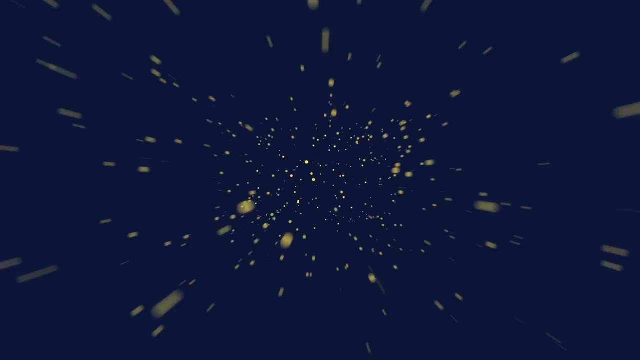 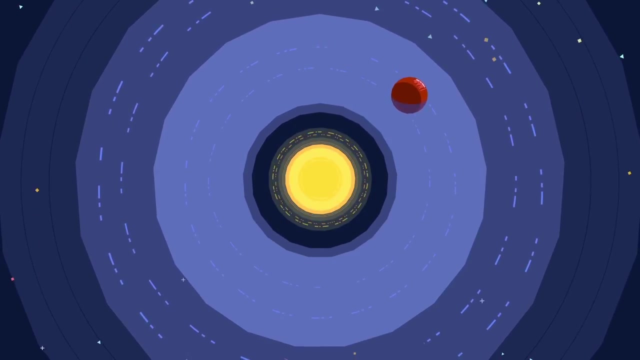 other than the Sun. Many of these extraterrestrial planets are in their star's habitable zone, a range of orbits also called Goldilocks Zone after the children's fairy tale. The little girl with golden locks hit the sweet spot when she found baby bear's porridge.